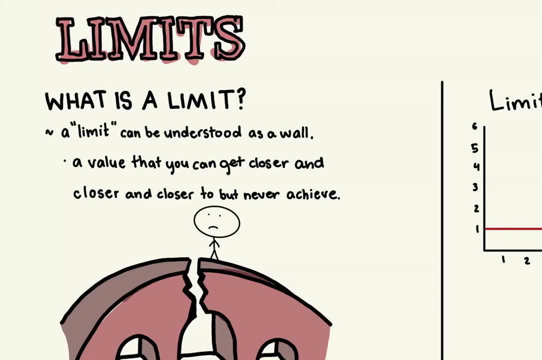 to be successful in the course, and just for math in general. So what is a limit? A limit can be understood as a wall, And it really just is a value that you can get closer and closer to, but you can never really achieve the value. Now let me explain what I mean, But before I do that, I'd like to explain. 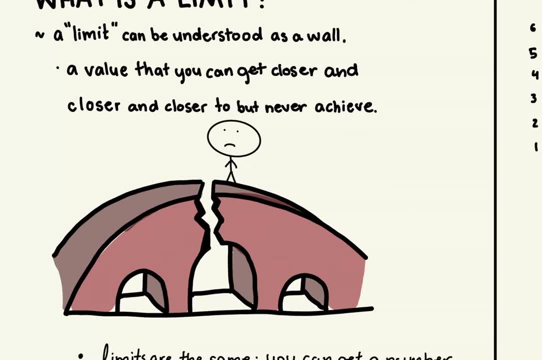 through actually giving an analogy. So imagine this: right here is you, Oops, Excuse me. Well, let's imagine this: right here is you And you're walking across a bridge And you find out that the bridge is actually broken. So you could walk closer and closer and closer to the. 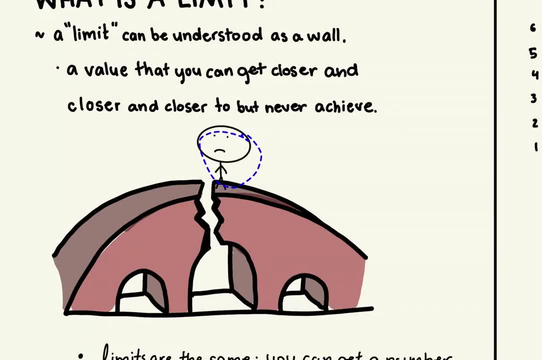 bridge And you can get so close, but you can't really stand in the middle where the bridge is broken because, guess what, you'll fall down. So you can get closer and closer- And that's really the same idea behind limits, because you could move in, you could move forward an inch or half an inch and even smaller. 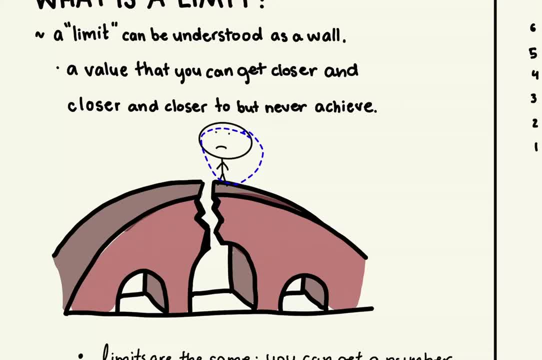 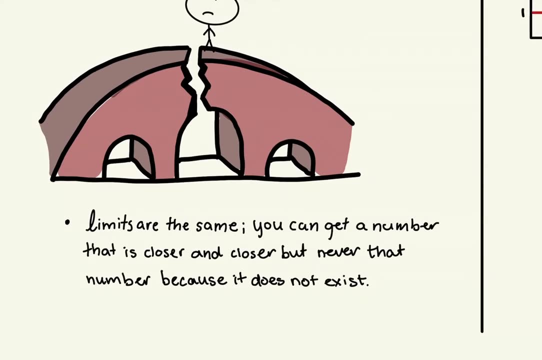 just small incremental values. you can get closer and closer to the, to the, to the crack, but you really can't stand there because there's nothing over there. And if you do stand you'll fall. So, similarly, the concept of limits suggests the same. you know, you can get a number that is closer. 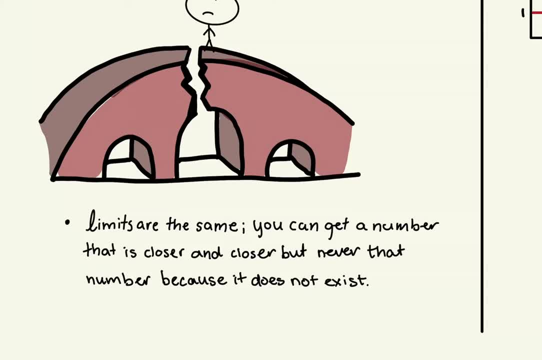 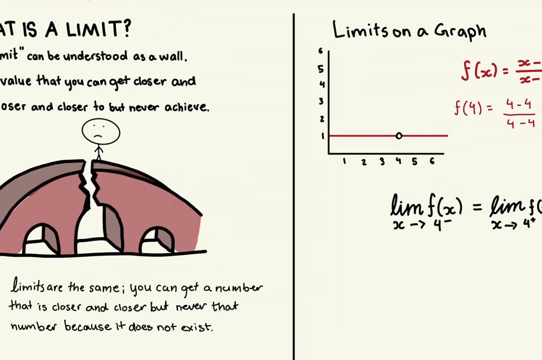 and closer, but never actually the value of the limit, because it just simply does not exist. As we saw, the, the bridge did not exist at that specific point, So that's why you would actually fall over there, And limits are just exactly the same And you can kind of see limits on a graph. So let's take 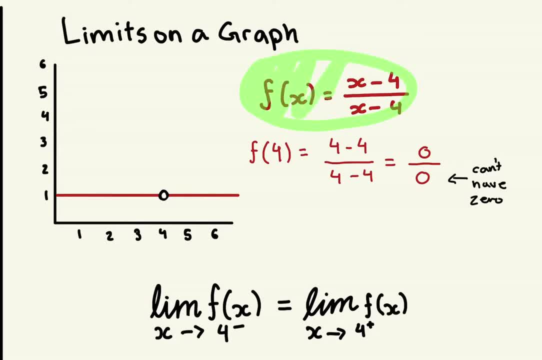 this equation right, or this formula right here, As an example, f of x is equal to x minus four over x minus four. Now you might think to yourself: you know, anything over itself is equal to one. So, for example, if you had, if you had five over five, that would be equal to one. So if you think to yourself, 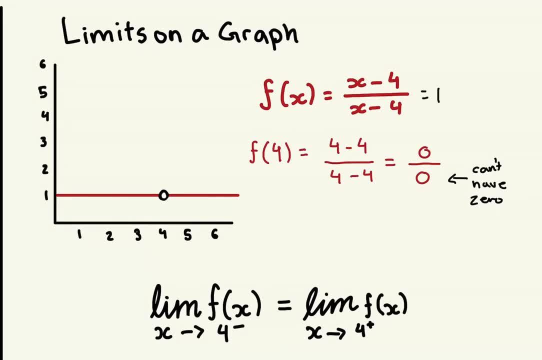 x minus four over. x minus four is equal to one. you would be right- except not really because you would- and consider the fact that if you were to plug in the value of four for x, what's going to happen is you're. 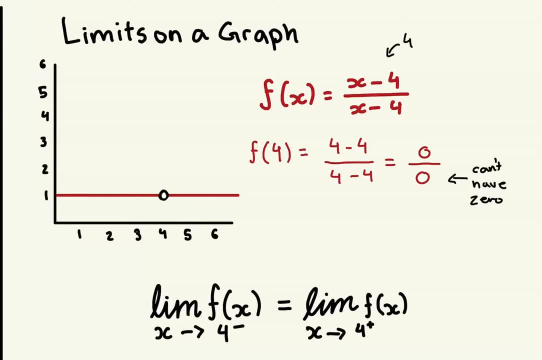 actually going to get four minus four, over four minus four And once you get zero in the denominator. that just doesn't work mathematically. So really this is equal to one, as long as you can add the exception that x is not equal four. So this kind of this kind of concept is really where the limit, kind. 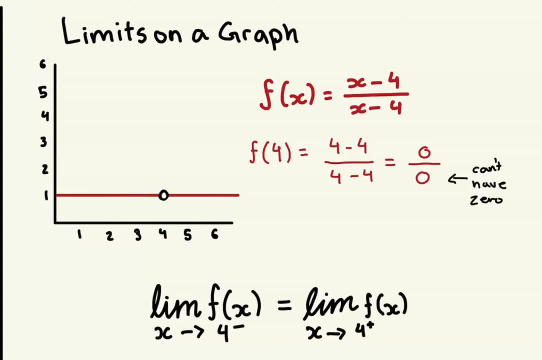 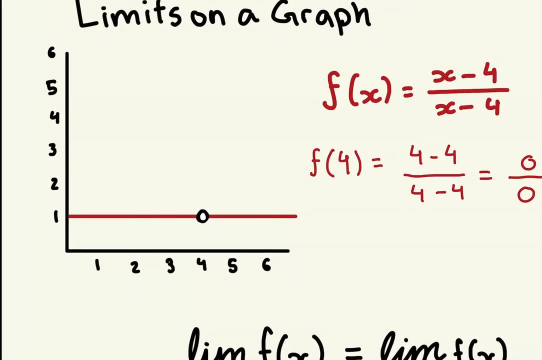 of comes into play. And if we look at this on a graph, which is the graph of this, of this formula or this function, it shows that it's the same thing as what I said before, where f of x is equal to one. So we see a straight horizontal line running through one, except at the 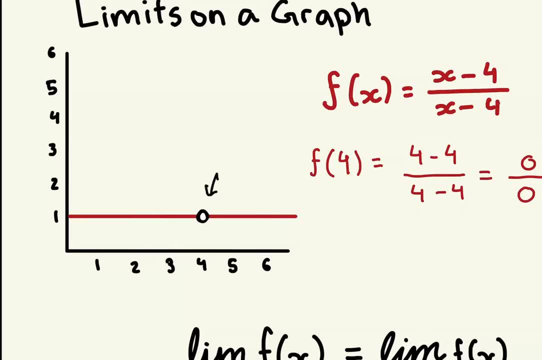 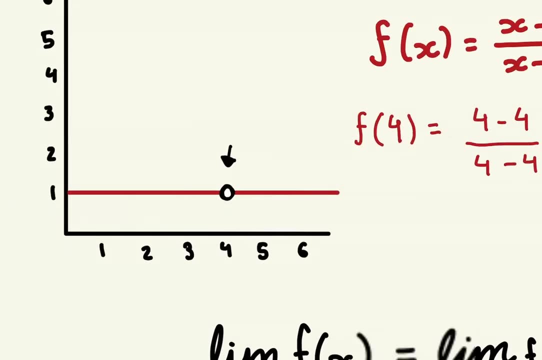 point of where x is equal to four And where what we see over here is that there is a discontinuity, And this discontinuity over here is is really where we'll see the idea of limits come to play. So what's going to happen is, you can see that if you approach, if you approach this specific value over here, if you 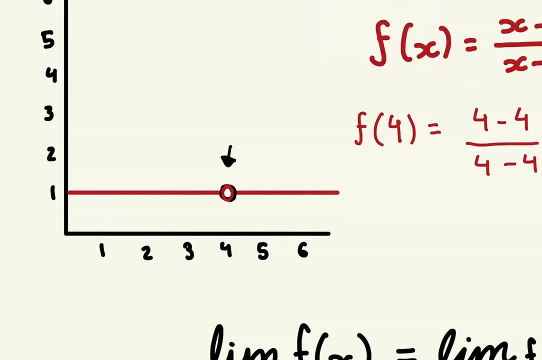 approach this place over here from there, from the left side, you're going to be approaching the v, so don't forget that the limits really are. whenever we talk about limits, we're referring to the y value, So the limit over here would be one. 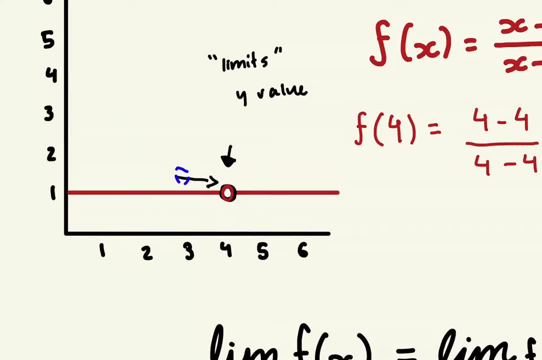 because as you're approaching from the left side, as you're approaching from the left side over here, you're going to be approaching the y value of one, And that's really the same for this whole thing, but it goes to show the same concept. And if 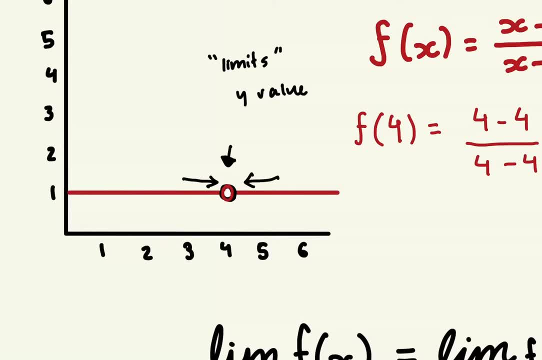 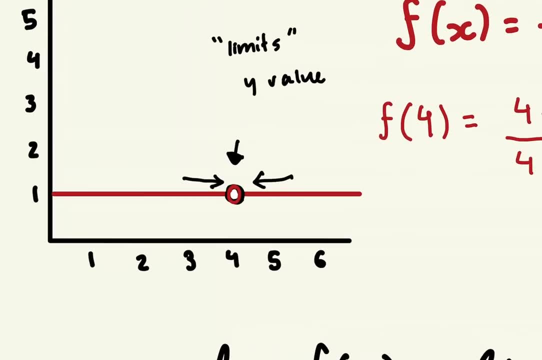 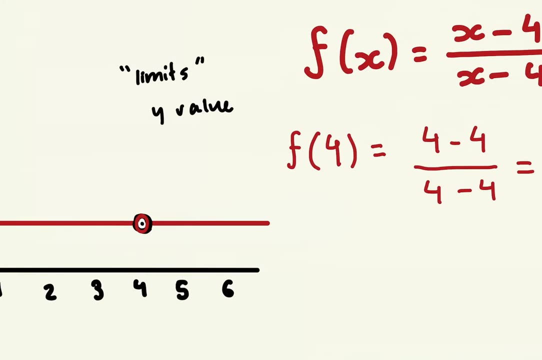 you're approaching from the right side, you're also approaching the same value, which is one, the same y value, And what's what's key to understand is that because this place does not exist inside this formula, as we saw over here, actually putting four inside. 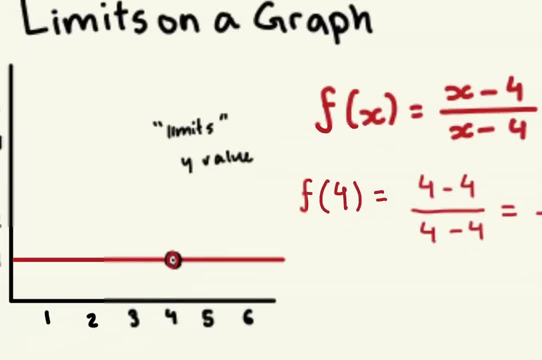 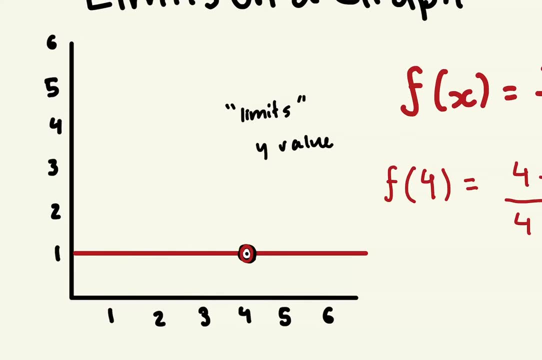 would make it would make it make it have a zero in the denominator. So that does not exist. It's a, it's a discontinuity, So you can actually have it equal to four. You can actually have the y value or the x value equal to four. because it's not defined at that point. This function is not. 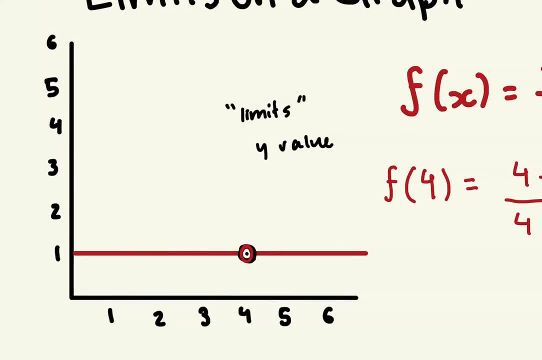 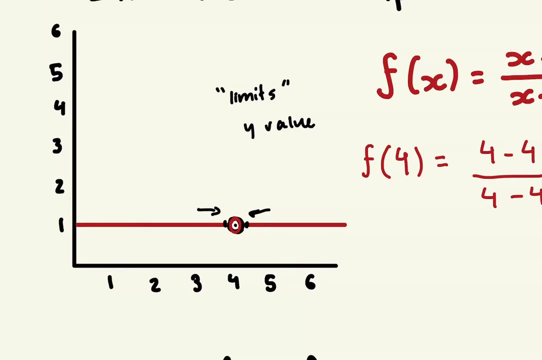 defined, but it is defined for any other value around four. So if we put in 3.9, or 4.1, it's going to give us one over here and over here is what we're talking about. So as we get closer and closer, no matter how close we are to four, it could be 3.9999, or really as many as you want you're going to. 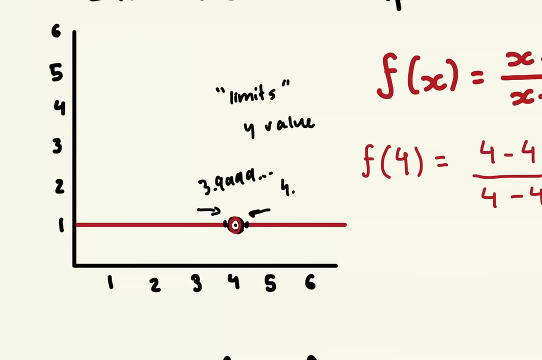 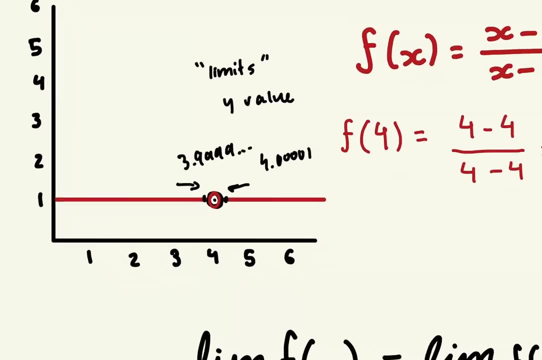 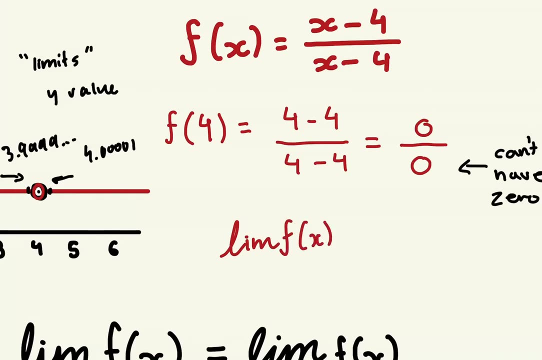 have a value of one, And you can do that from this side as well. you can do 4.00001, you still don't have a value of one. So that is the limit over here And the notation for that is the limit of f, of x, which we're referring to, this equation right here. 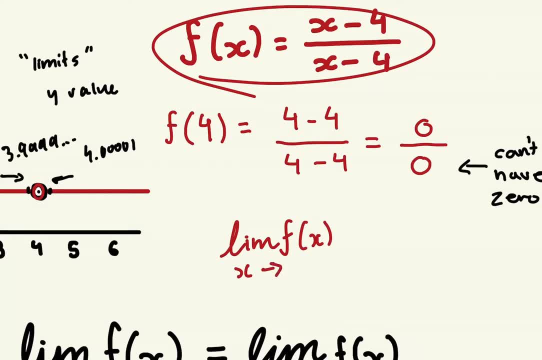 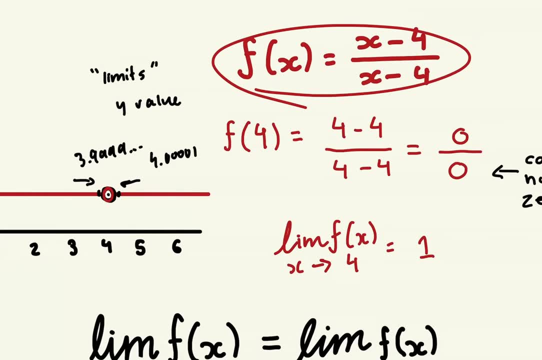 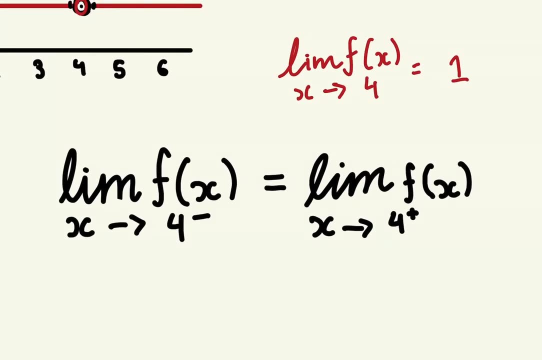 As x approaches whatever value we have over here. it's four And that limit is as we discussed earlier: it's one. So when actually figuring out limits, there's one key thing to understand is that the limit actually has to be the same from the left and the right as we were. 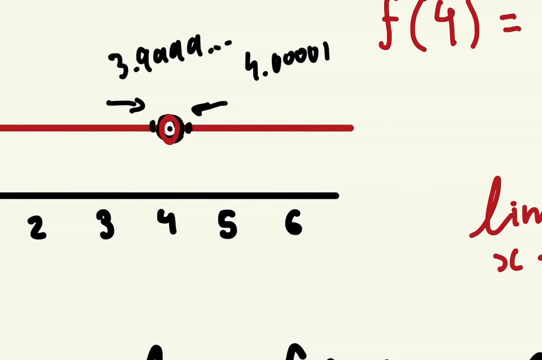 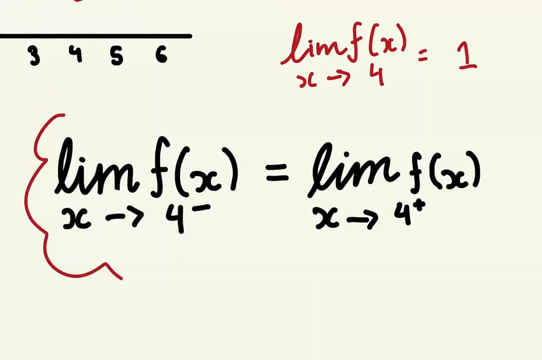 talking about earlier. So if you look over here, it's approaching the same y value of one from both sides And that's that's really important for a limit to actually exist. And this is this complicated looking thing right here. for someone might actually be really simple, because that's really all it's saying. It's just saying that the limit 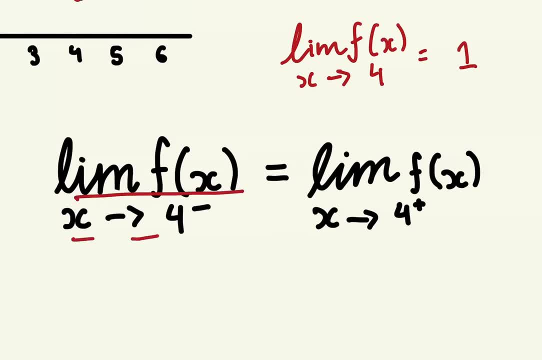 of f of x, the limit of f of x as x approaches four from the left. so this negative just signifies from the left is equal to the limit as x approaches the limit as x approaches four from the right. And basically what's that saying is: you can't really have. So if we actually 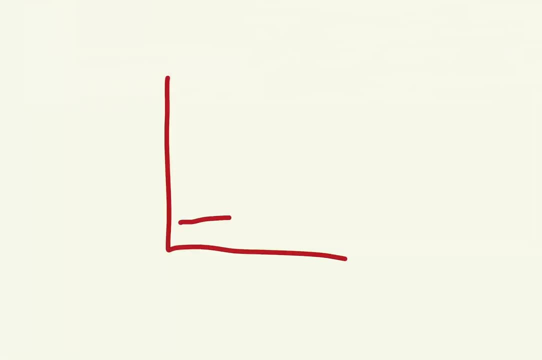 were to have a graph over here and you can't really have a limit looking like this, All right. So if you kind of had a graph like this, you could say that the limit as f of x, so this respective function, x as limit of f of x, as x approaches. let's say, I don't know three approaches, three from the left, is equal to one, because that's.